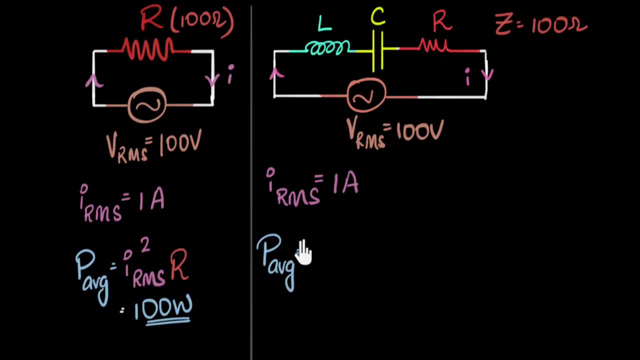 just like earlier here, average power might be IRMS squared times total opposition, which is Z. Let me use red for that Z and we might think, okay, maybe we end up with the same answer, which kind of makes sense, right. 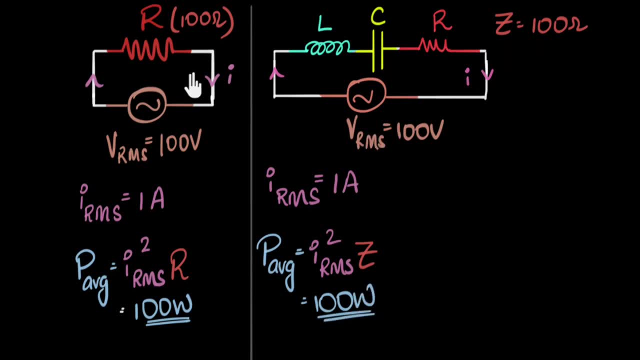 Because I have the same voltage, same current, same opposition as before. everything is the same, so maybe the power distribution also remains the same. But this is not true. This is wrong. Why this is wrong? Why? Because the entire opposition does not. 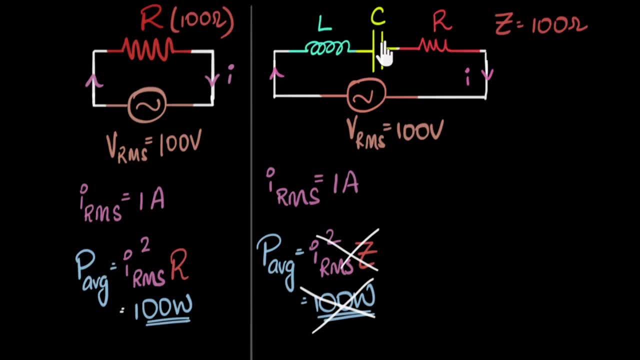 consume power. Here's what I mean Among LC and R. the resistors consume power, just like before I square R. but what about the inductors and capacitors? They do not consume any power. For example, if you tell a capacitor 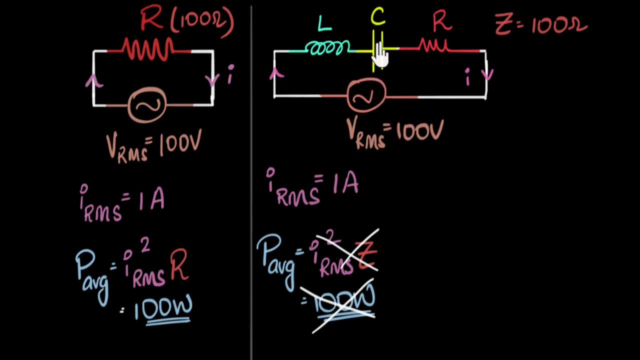 then what you'll find is, when a capacitor is being charged, it definitely consumes power. It stores energy in its electric field, but then, when it gets discharged, it transfers the power back to the source. Therefore, on an average, that's almost zero. 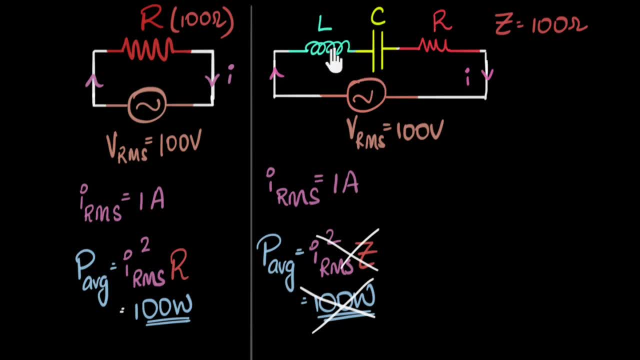 it does not consume any power. and same is the case with an inductor as well. on average, it consumes zero power, which means the entire opposition, the entire impedance does not consume power. only the resistive part of it consumes power, which means even in this circuit, even in this circuit. 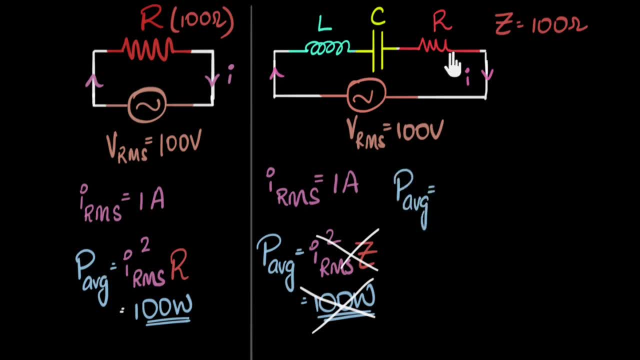 the average power consumed would only be the power consumed by the resistor. so it will still be. I rms squared times R, and so would it be the same as before? no, because before the entire resistance was 100 ohms. this time the total impedance is 100 ohms and therefore resistance. 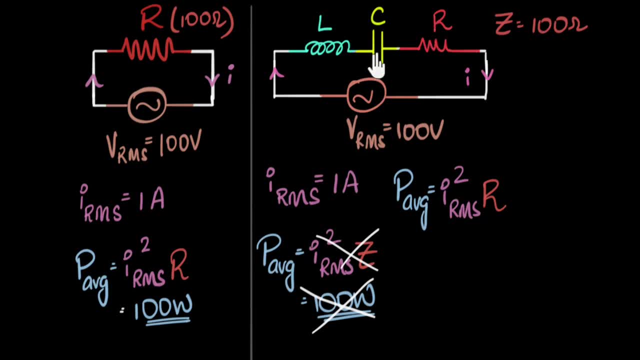 would definitely be less than that. now, how much that depends upon the details, we don't know. but let's say for the sake of, for the sake of some example. let's say the resistance in this case is just 10 ohms. that's totally possible. maybe the reactances are very high. 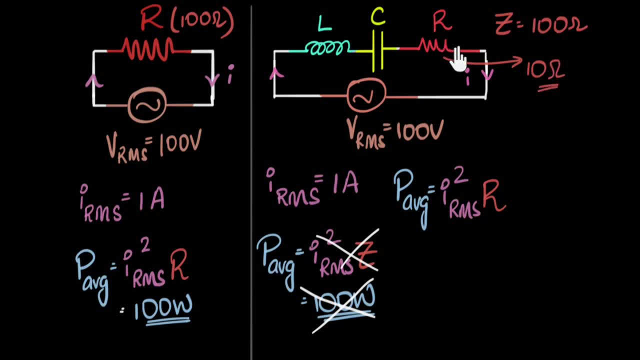 and, as a result, I'm getting total impedance to be very high. it's totally possible in this circuit that I can have resistance to be only just 10 ohms. then, in this particular example, the average power that gets consumed by this circuit is going to be 1 square times 10, which is going to be just 10 watt at first. 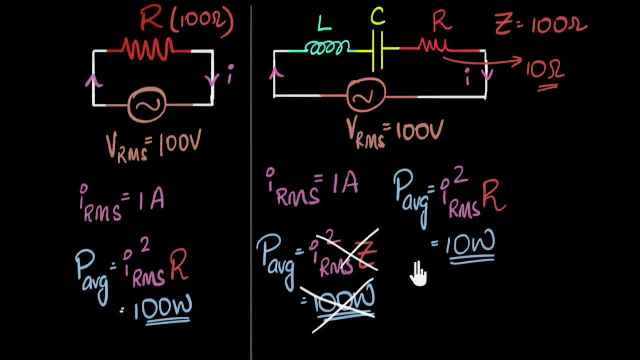 this did not seem like a big deal to me. I mean: smaller resistance, less power consumed. larger resistance, more power consumed. so what's the big deal? this is where the electric company calls me and says: oi, Mahesh, you are consuming the same voltage as before, same current as before, yet you're consuming way less. 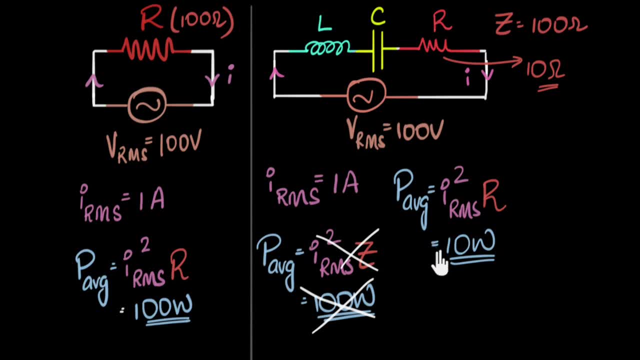 power than before. and I say yeah, so what's the big deal? the big deal is- and this is where the electric company is trying to explain to me the problem- see, when we are delivering electric, whenever electric current is passing through our transmission lines, it gets heated up, so there's some energy loss happening, right? 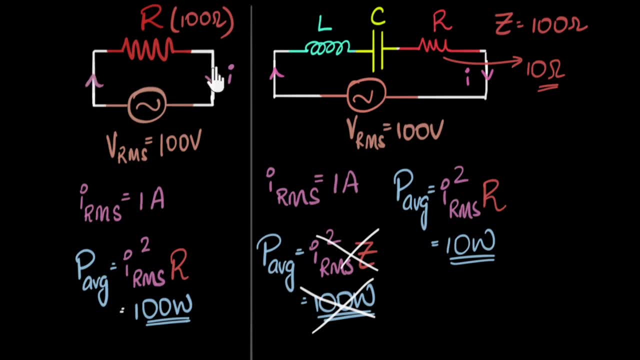 who's gonna pay for those energy losses? let's say that energy loss over here was, I don't know, maybe 20 watt. now when I'm consuming 100 watt energy loss of 20 watt, the electric company might say, fine, not a big deal, don't worry about the 20. 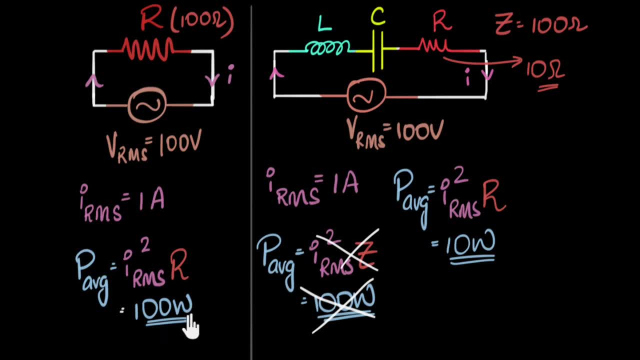 watt energy loss happening. you're, you're consuming 100, you're paying for that. it's compensated. I have enough profit margin. but over here the energy loss stays the same because the current is the same and the voltage is the same. so the energy loss here is 20 watt. I'm only consuming 10 watt. so the electric 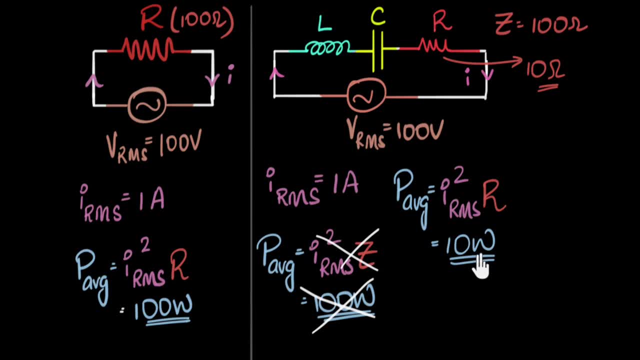 company says you at this time it's not, it's not profitable for me. there's so much energy, that loss that is happening just for your twin 10 watt of consumption. and so the person says: you have to pay more over here, you have to pay for my losses also. does that make sense? well, I'm sitting here, I'm thinking: 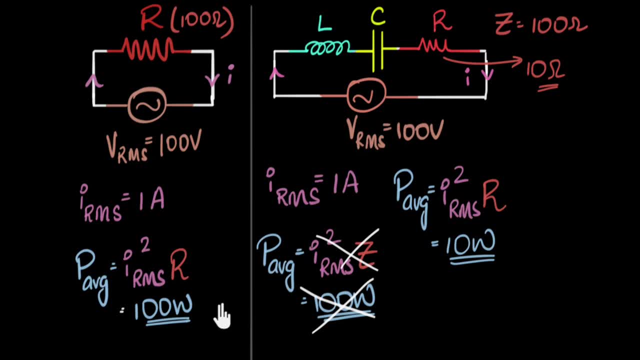 that kind of makes sense. it's kind of like delivery charges. when you're ordering something big and you're paying a lot of lot for it, then the petrol charges, delivery charges, are covered because they are small compared to how much you're paying. but if you're ordering, say, a five rupees pencil, I'm just 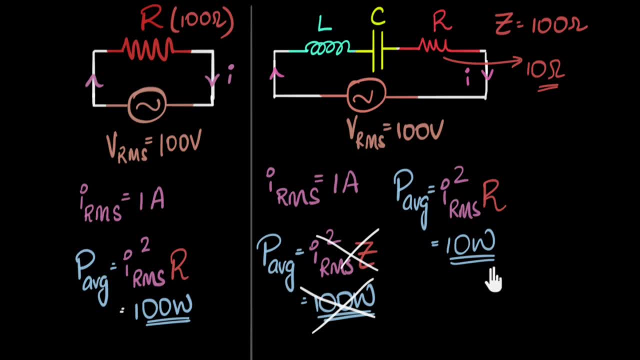 exaggerating, then you have to end up paying for the petrol charges and you have to pay for it. so from a power consumption point of view, this circuit has less efficiency compared to this circuit. right, because for every watt that you're consuming here, the energy that is lost, that is happening, is much. 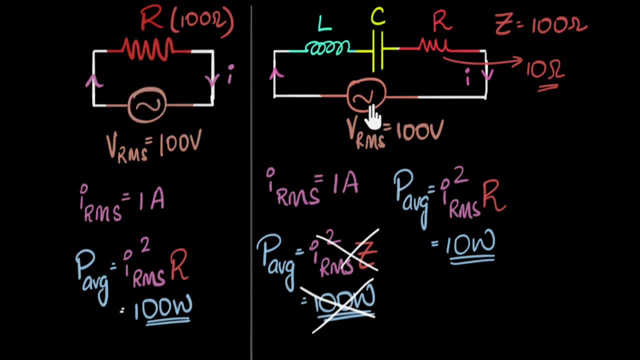 higher compared to over here. so immediately you might be wondering what do we do about it? well, the first step is to actually put this in numbers. when I say the energy of the power consumption efficiency is smaller, how do I like sort of represent it officially? well, to represent it, what we can do is we can. 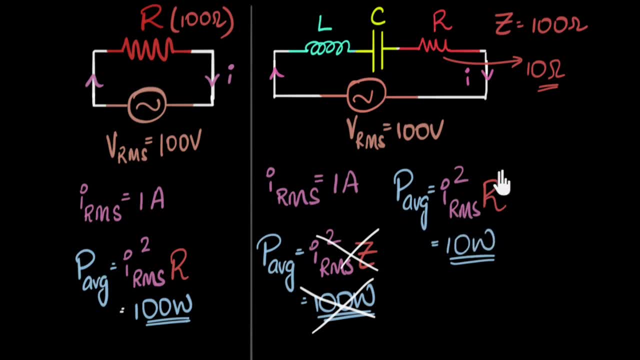 say that we can write this in terms of z. okay. so let's say, we can write this in terms of z, so we can write this in terms of z, so we can write this in terms of z. okay, and we can write this in terms of z, okay, and I want you to again give a shot. 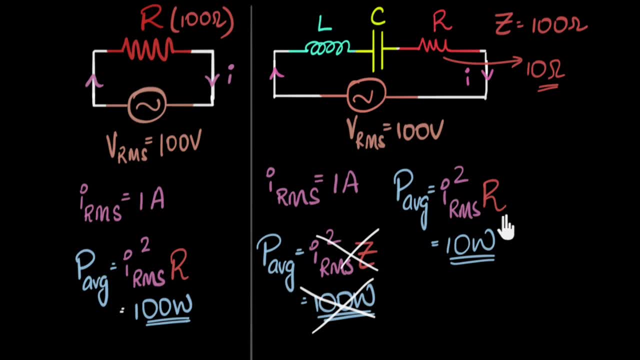 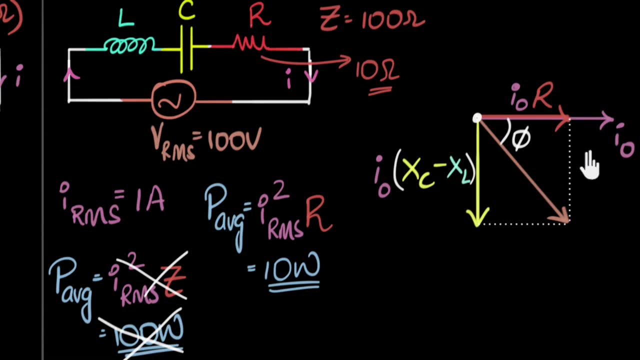 to give it a shot. how can you write the power dissipated in this circuit not in terms of R, but in terms of Z? how do you bring Z into the picture? well, I can help you a little bit. we can bring back the phaser diagram that we have seen before. 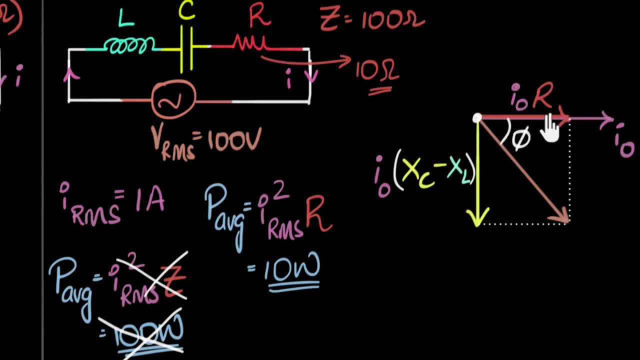 just to quickly remind you, I not represents the current, then the voltage across the inductors and capacitors are 90 degrees out of phase and if we are assuming that the capacitor reactance is larger, then the voltage becomes 90 degrees behind the inductor and then 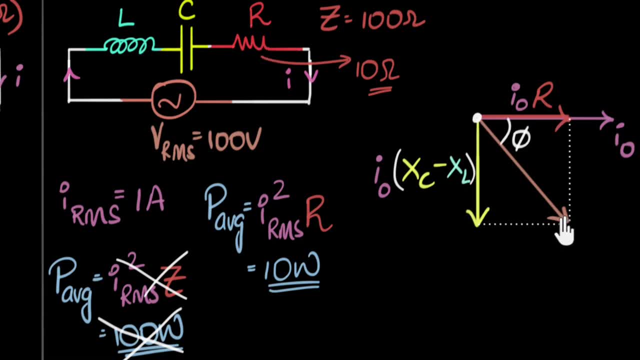 if we add the all the voltages together, we get the total voltage and we can now say that total voltage, we can represent it to be I0 times Z. right, you can, we can represent it this way. so what we can do now is we can look at this triangle and try to find the relationship between R, Z and Phi. 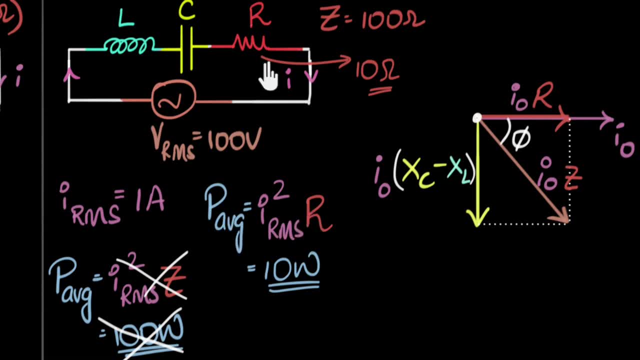 and then substitute over here to get power in terms of Z. so feel free to pause and try, all right. so since I want to connect the adjacent side and the hypotenuse, I'm going to use cos, cos Phi. is this divided by this? I not cancels out, and I end up with R divided by Z. and since, 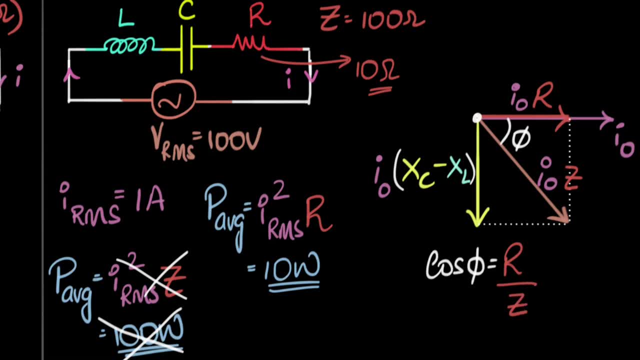 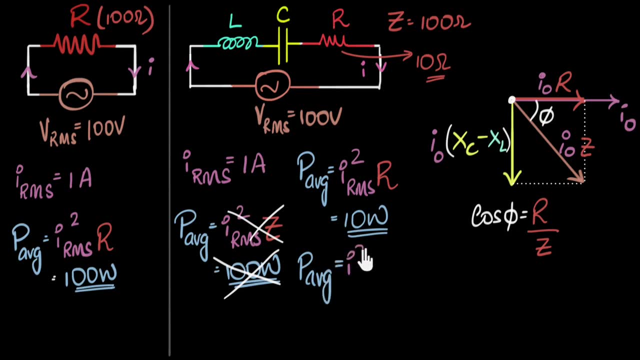 I want to substitute for R. I can say: R equals Z times cos Phi and as a result, now I can say: hey, average power therefore equals I RMS squared times. instead of R, I'll say Z, impedance times cos Phi. so this is the same expression as this you'll. 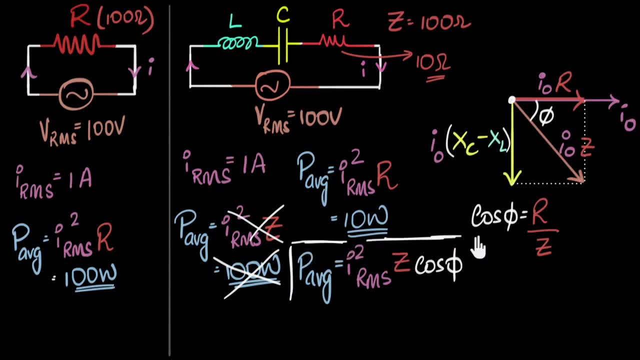 get 10 watts itself. but now we are representing this in terms of the total opposition, and this number, cos Phi, tells me how poor or how good my circuit is when it comes to power consumption, and so this number is called the power factor. okay, let's dig a little deeper for a pure resistive. 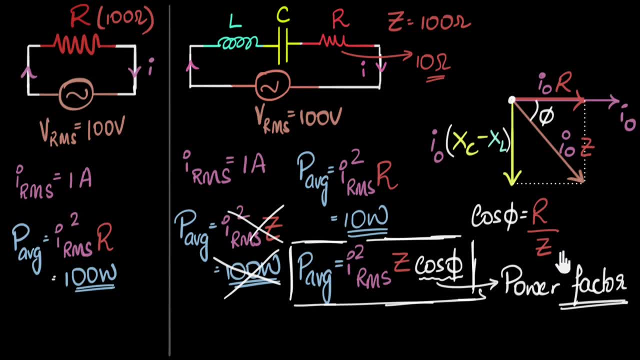 circuit. can you think about what the power factor would be? well, here impedance is equal to resistance, so Z is the same as R, RR cancels and you get power factor to be one. so over here, power factor is one. another way to think about this is we could say: hey, current and voltage are in phase with each. 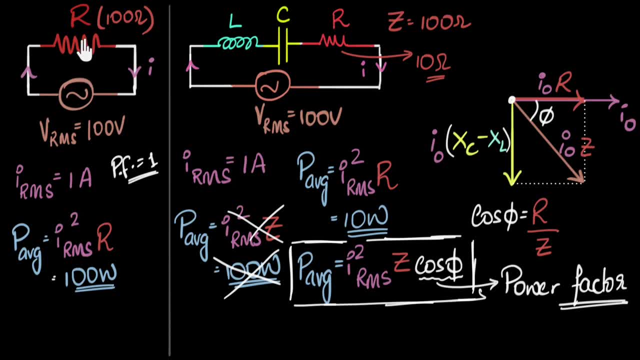 other. so, cos zero is one, you get the same answer, and so this means you get the maximum power consumption. your entire impedance is consuming power, because your entire impedance is just resistance. okay, what about circuits that only have inductors or capacitors, no resistors at all? what? 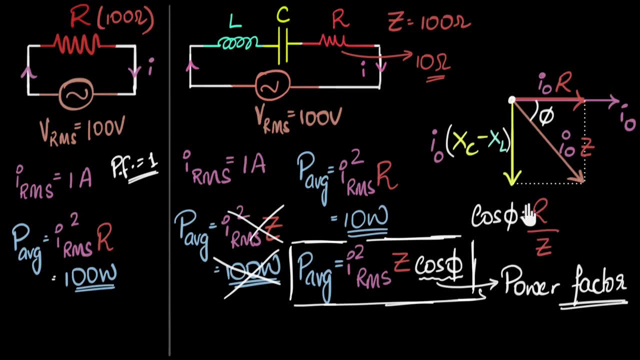 would be the power factor there. well then, R is zero, power factor becomes zero, and that kind of makes sense, because we just said that inductors or capacitors, on an average, do not consume any power. so here the entire impedance is not consuming any power, and so since there is a current running over, 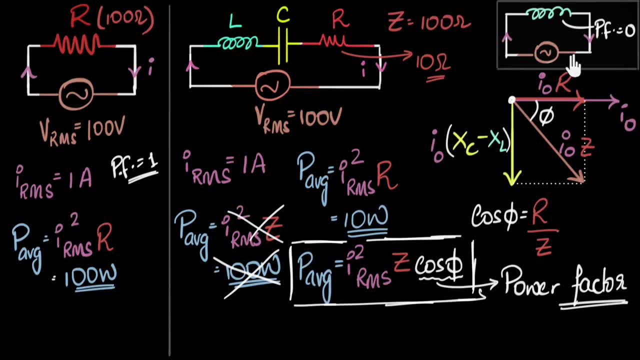 here. but but there is no power consumption due to that current. we call these currents watt less current, watt less current. and from an efficiency point of view these are the worst because there will be a heating effect in the transmission lines. there will be energy losses, but for what you're? 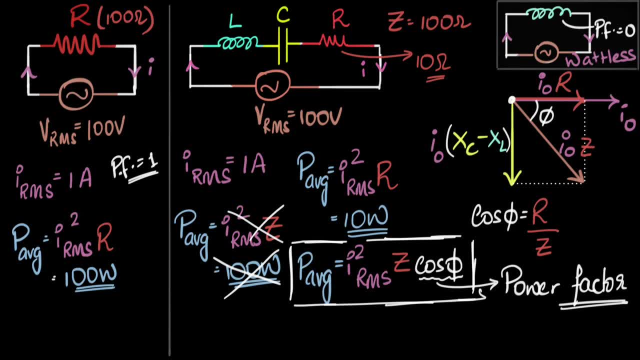 not consuming any power. so this is, this is the worst circuit you can think of now. of course, real circuits will always have all components, and so their power factor will always be somewhere between zero and one. the closer it is to one, the better. it is better efficient it. 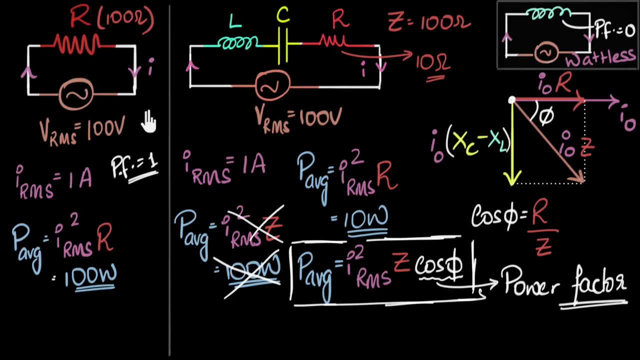 is when it comes to power consumption, and you can now also appreciate why we like resonance here. we have seen before that at resonance the impedance is pure, resistive, and therefore at resonance the power factor is one, and so if you're consuming power at resonant frequency, then you 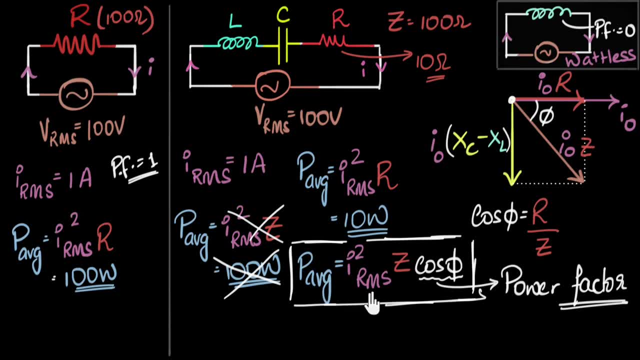 will be consuming the maximum power. okay, I want to end this video with a question. what if we have an LCR circuit whose LCR and the frequency values are all fixed and it has a very poor power factor? what can you do to improve the power factor of that circuit? 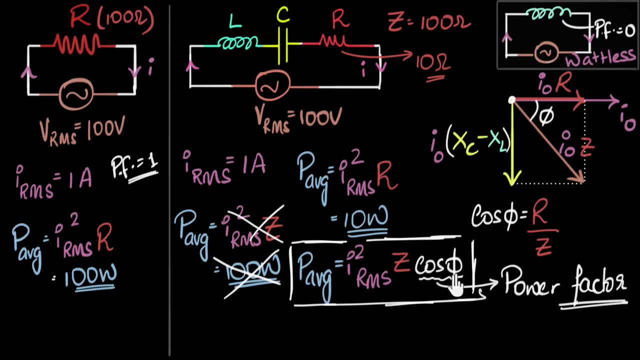 I'll give you a clue. if you have poor power factor, it means the Phi value is very large. it means the phase difference between the voltage and the current is very large. so the question is: how can you reduce the phase difference without changing this? but you can also reduce the phase.